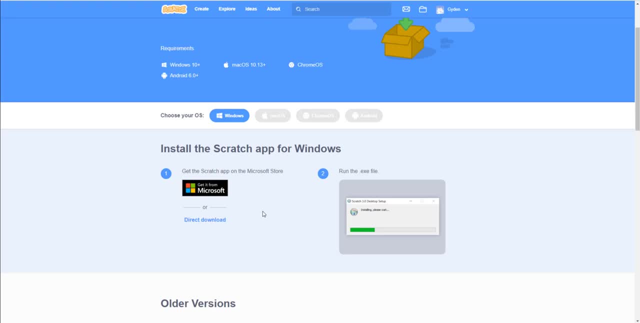 meaning you can actually run it anywhere. But I do recommend the online version so that if you have online access then you can pretty much use it anytime. The offline versions, you know you have to save it locally on your file and you have to like load it up. But 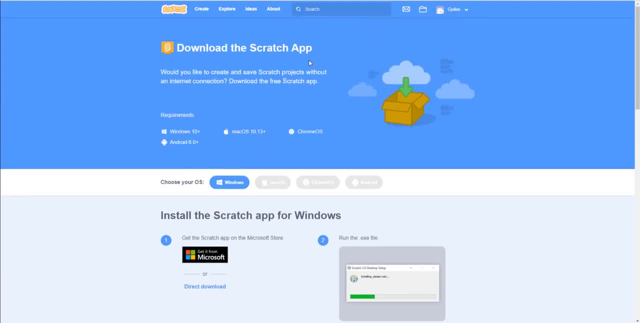 it allows you to work online without internet access. But the online version, everything is saved into your project. So let me get started. So now that you have a little bit basic of about Scratch, where to go and how to download the Scratch and how to log in, 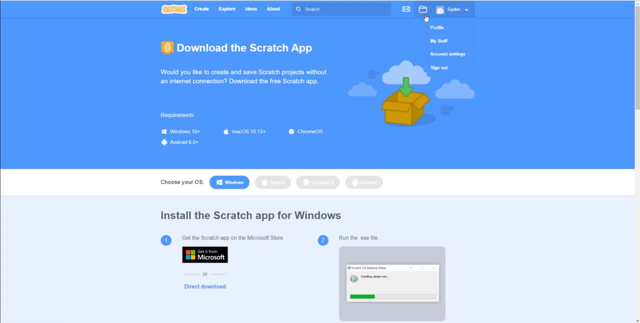 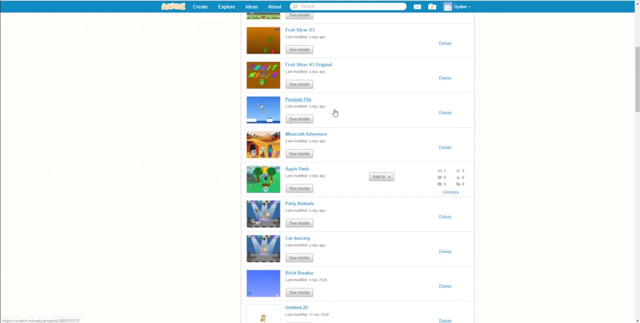 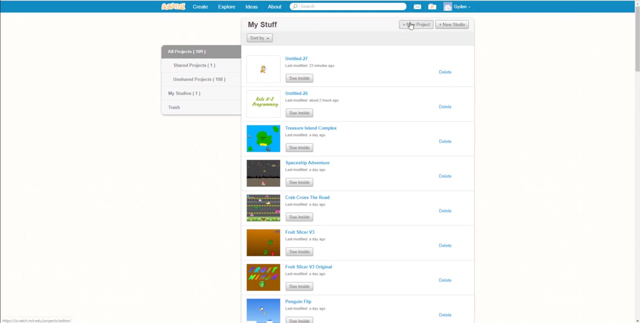 and use it. So once you log in you'll see you can go to my stuff. click on this and it will show like different stuff, what are some of the projects you have for Scratch, So you can also create your new project. So we can do that by clicking on this button. 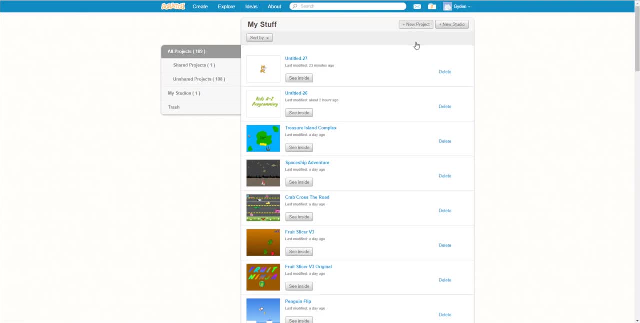 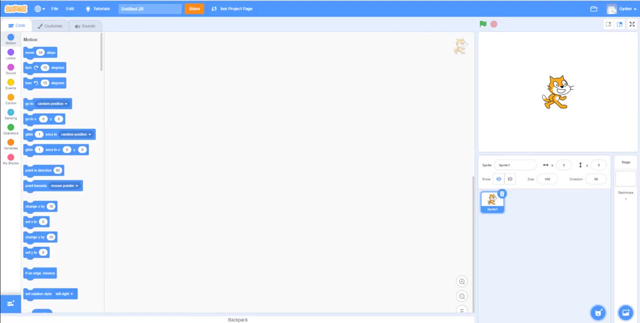 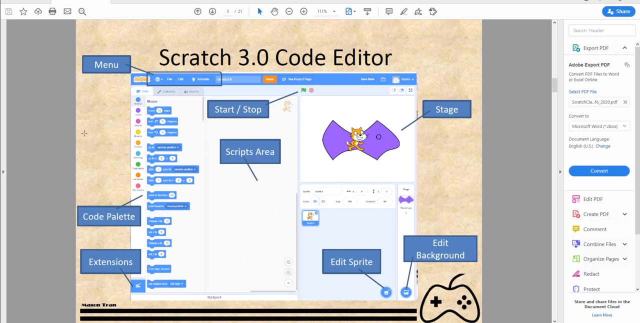 here create new project. So when you create this new project it will load into this editor. So this is the editor for Scratch. Okay, So let me show you one of the slides I made about the Scratch. So here the Scratch editor. 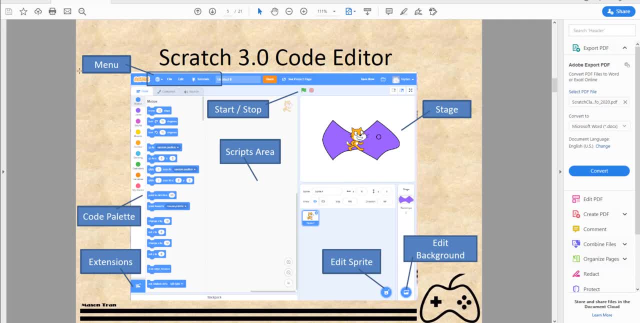 this is a 3.0. Scratch recently updated to 3.0. So this is a menu. So this is the menu bar you have here. This is the stop and start. This is the button to run your game. This is the script area where you put your code. here those blocks. This is the code palette. 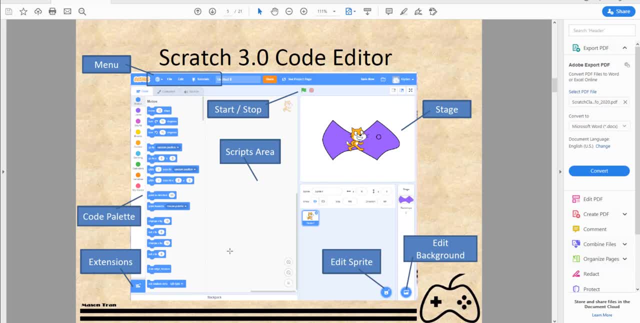 So you can drag and drag the code and drop it into the script. This is the script area And these are the extension. Extension is like other stuff, like music pen, you know, or other things that you want to use with Scratch And this. 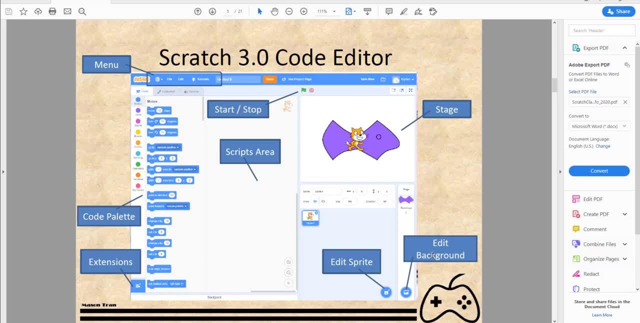 is the background editor. You can put a background for your game. This is the sprite editor, where you can edit, put in different sprites, like the cat. here, for example, You can have a dog or something else. And this is the stage, meaning like what you're going to see. So 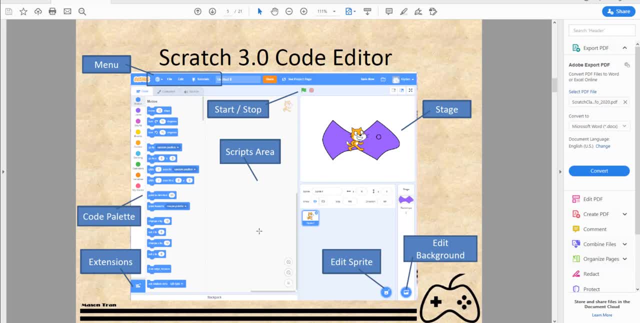 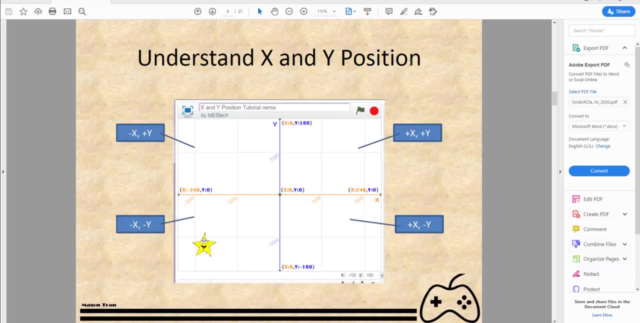 you're going to be able to create your own game So you can see how your game runs. So this is the basic of the layout for the Scratch. Next, we want to understand about the X and Y position of the Scratch. So in the center of Scratch will be 00.. This side. 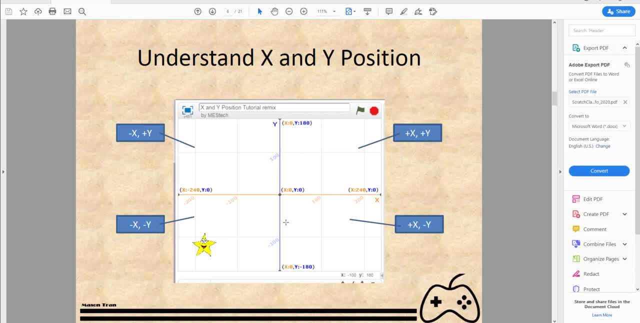 will be positive X, right, This side will be negative X and this side is positive Y. This down here is negative Y. So, as you can see this quadrant, here is positive X and positive Y, Here is positive X, negative Y, Here is negative X, negative Y And here is negative X, positive. 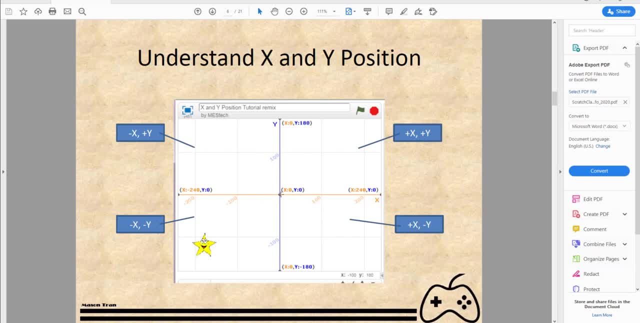 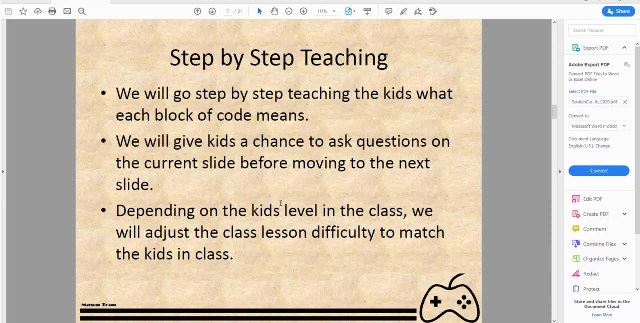 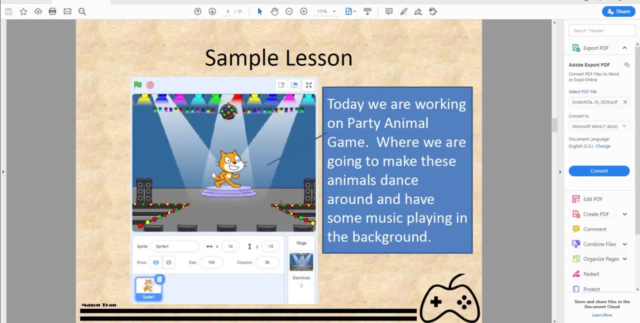 Y. So you have to kind of understand the position. So 00 is kind of in the center of the stage, Okay, So next we're going to go step by step teaching the kids how to code the first Scratch game. Okay, Here we go. So this is the sample lesson we're going to work on today. So we're 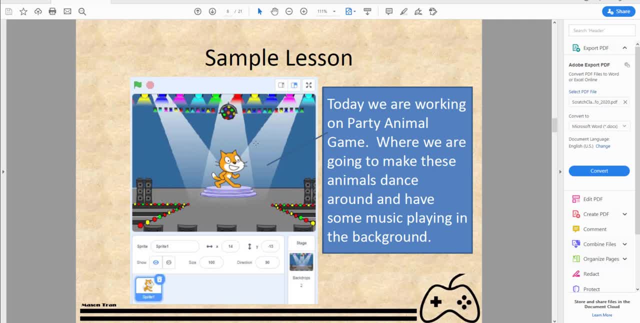 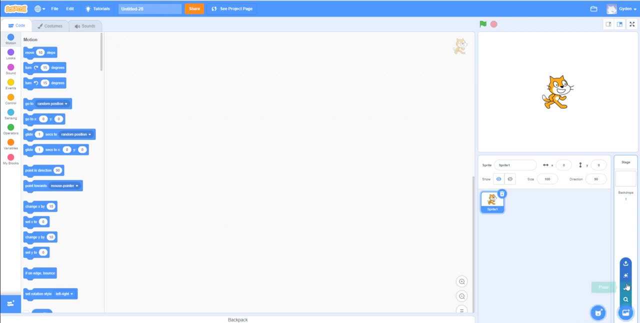 going to have the cat in the background with the music and the cat will be dancing. Okay, So let's start with the program. So first we have the cat right. So what we can do is we can click on this button here and go into here, say select the background and 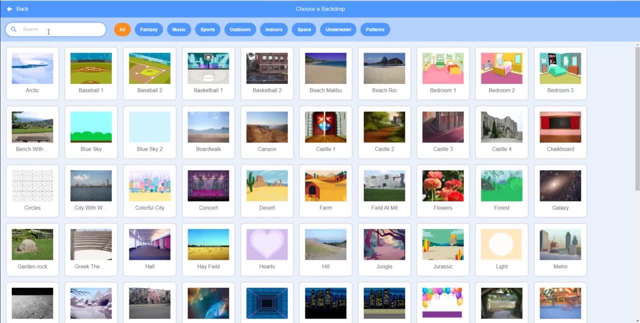 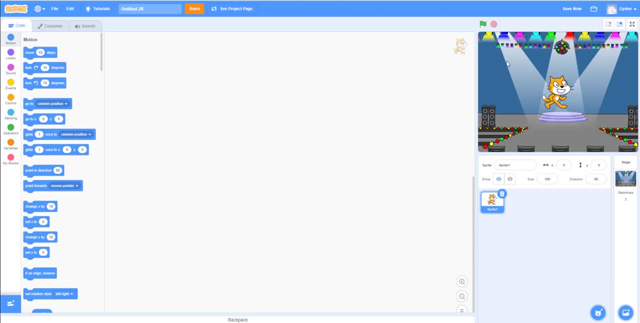 then you can type, maybe dance. let's say, Yeah, see, dance. So you have this spot here, spotlight, select this. So now you have the cat, have a background of the dance stage. We're going to move the cat kind of in the middle of the stage here. So after that, what? 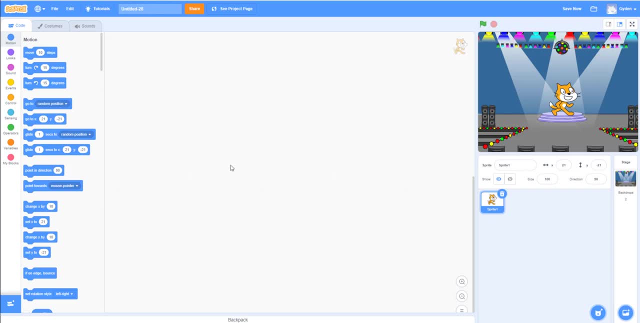 we can do is we can do some coding to make this cat move. So first thing we can do is- you can see these here. These are the different code block they have, So we can start with the first one events. So when the button is clicked, what do you want the cat to do? 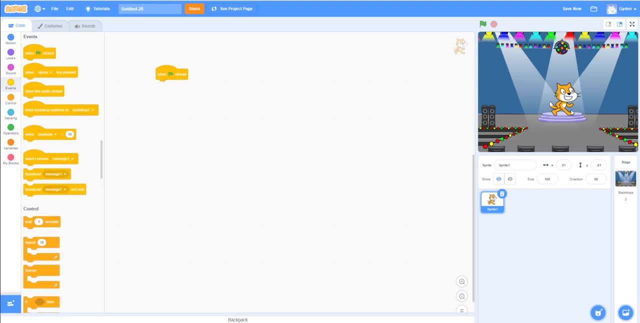 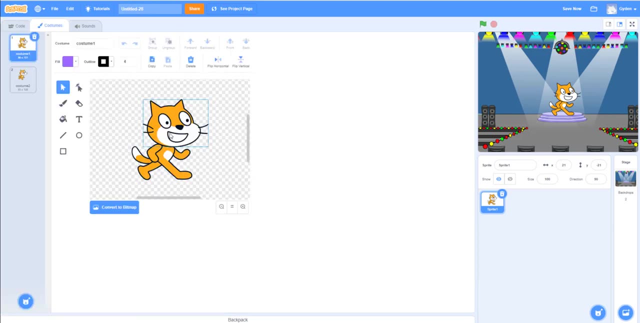 So the cat is not doing anything right now. Let's say, we want to make the cat move, So we're going to have to take a look at this costume. So, as you can see, the first costume is the cat kind of standing here. Second costume is the cat kind of like moving his leg. So 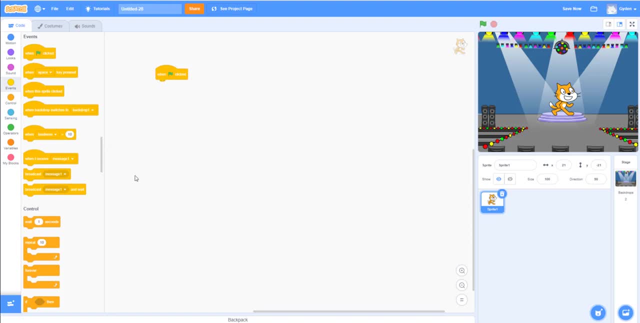 you can. what you can do is you can put a loop. We'll go into more detail on this later on. Just follow along So you can see here control. We can drag this for loop into the, into this block here. So it was kind of like a Lego kind of thing. You slap, snatch it in. So 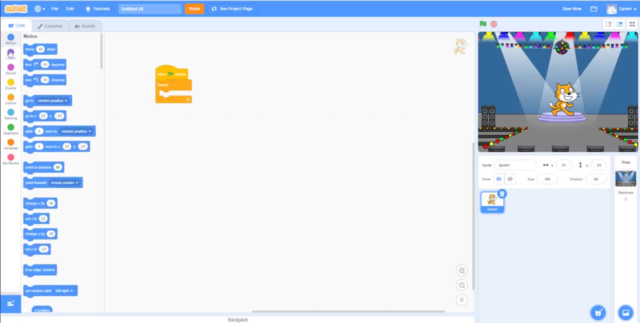 and then you can say: go back to here, look and look. you can say next costume. So what you do is when you click on this, you will see the cat continuously forever changing the costume. So I can click on this Once, So you can see it kind of going really fast. right, That's what we're not, not what. 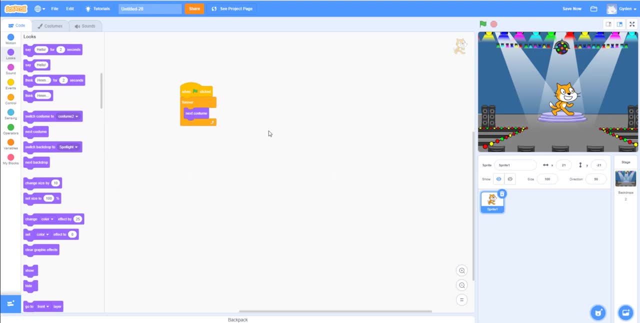 we want, right, We can stop it. So what we can do is you can put a little bit of weight, Okay, In the control. I believe Yeah, Let's see Yeah Here. So you can drag weight over here. You can do like 0.1 second. So this is like a fraction of a second right. So 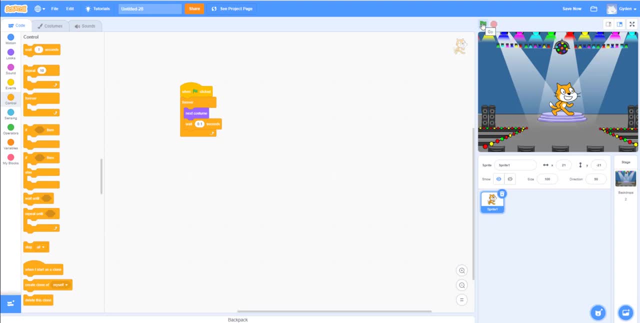 let's say, if you go start again so you see how you click on this green flag goal, That means they will execute this block of code Here. So let me kind of zoom in so you can see better. I should do that earlier, Uh. 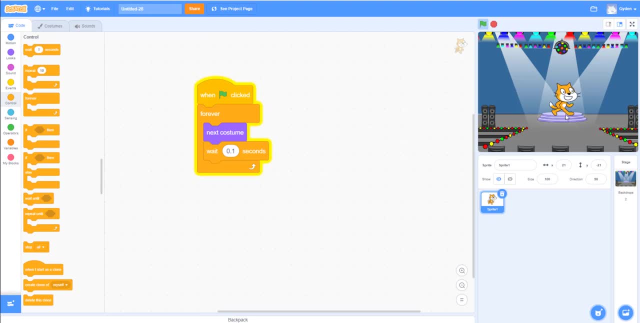 so now let's, let's click on this goal So, as you can see, you can see the cat is kind of running or dancing or what it's doing, And you can see that this block of code has become yellow, meaning this is running, so you can stop this. Now we have the cat moving. 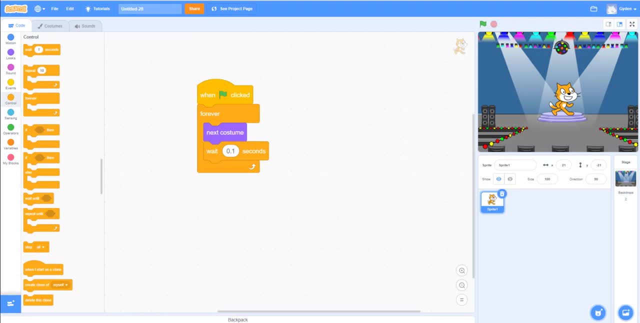 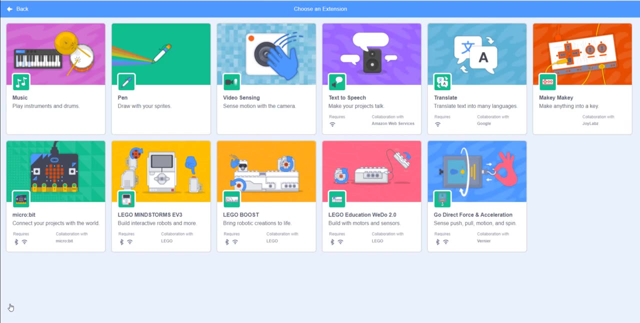 kind of thing. So now let's say we want to add some music to the cat, right? So what we can do, uh, we can, Okay, Go in here and then we can. this is the extension. We can add music extension. So once you add, 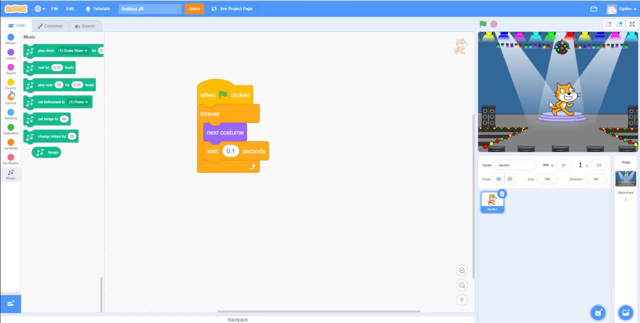 the extension of music. you see something like this. So what we can do is we can go back to the event. We're going to drag another uh start when start is click, And then we are going back to the control. We had another uh forever loop here, And then what we can, 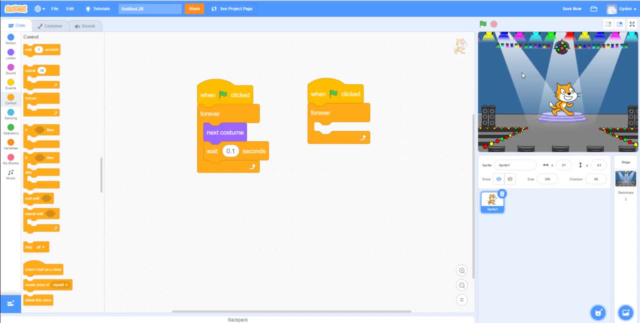 do is we're going to make the cat kind of moving, Uh forward a little bit, moving back a little bit. So this is a movement, So you had to go to motion. So you can say, uh, move forward, 10 step, And what we can do is go back to. 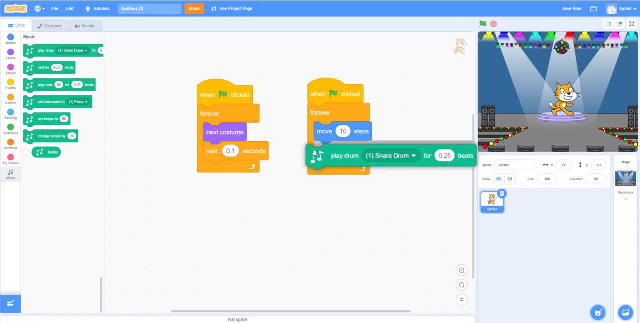 the music We can say, Hey, play this drum, sound right. Or uh, 0.5, two second for the beat and then play and then make the movement again, And then we can use like uh, moving back right. 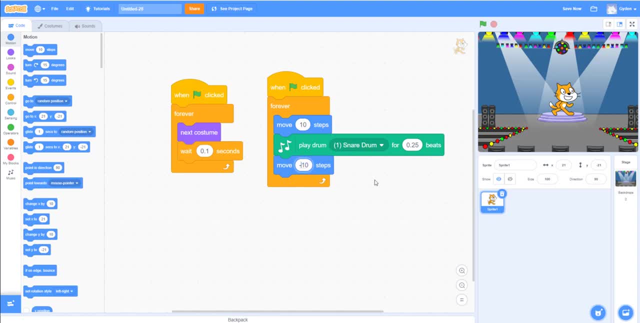 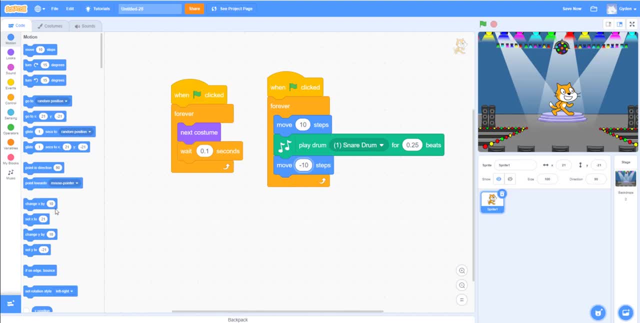 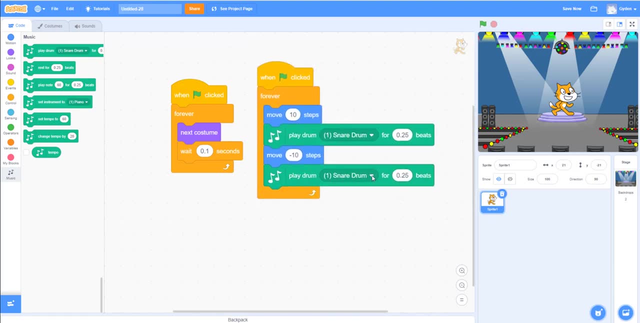 plane is moving forward, I'm moving backward, and then we can use another music, like, let's say, can put another sound here and you can choose a different sound. Maybe you can choose this one, Right, And then you can also make a move forward again, or you can just duplicate. 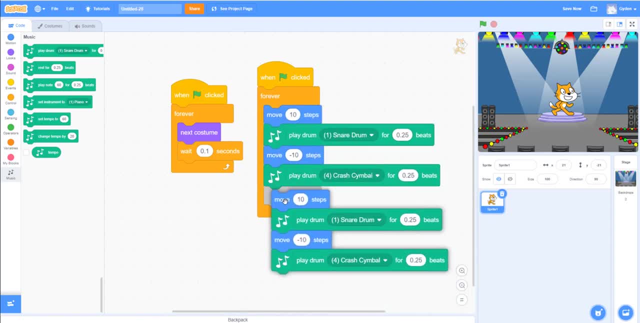 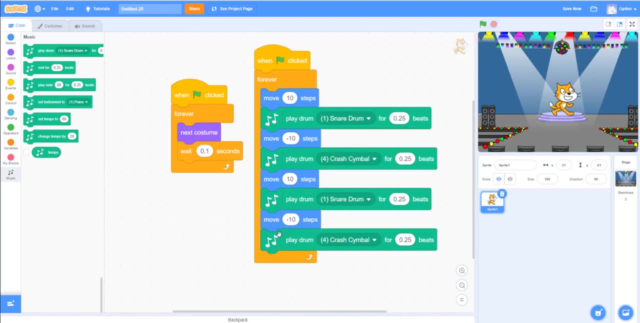 a code, Right click, duplicate. All right, So now you have a second set of code so you can see it's playing some sound. we can move backward and forward again, and then maybe we can delete this part. we'll only drag it. 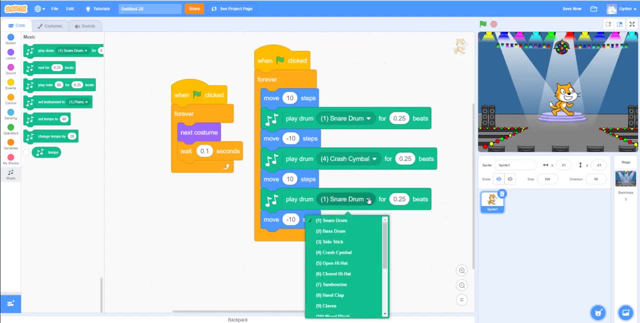 back in here. we'll delete that, This one. we can just select another one here. So what happens? if I run this code now, you'll see that the cat will continue moving, dancing, moving forward and backward, and then we're changing the costume and playing this sound. 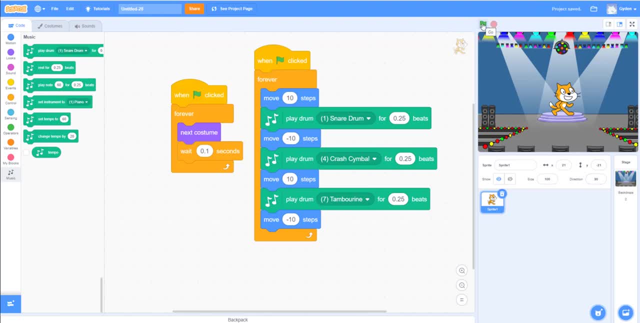 So let me run this real quick. we'll save our project, we'll run. so you can see the cat is kind of dancing like this: forward and back, forward and back right. So, as you can see, this is a really simple project we created so where you can make. 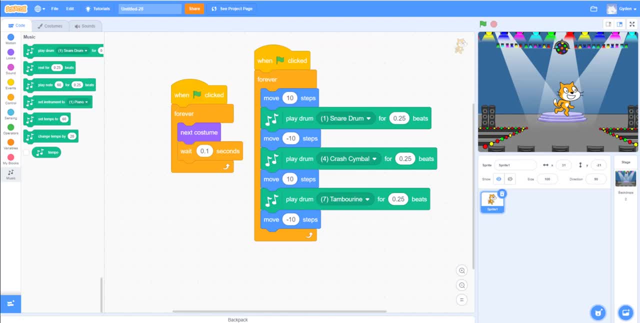 the cat dancing, right. So next, what we can do is we can also make the cat maybe change in color. So there's another event you can use. right, different event, let's go back to the event. So when space keeps changing, right. 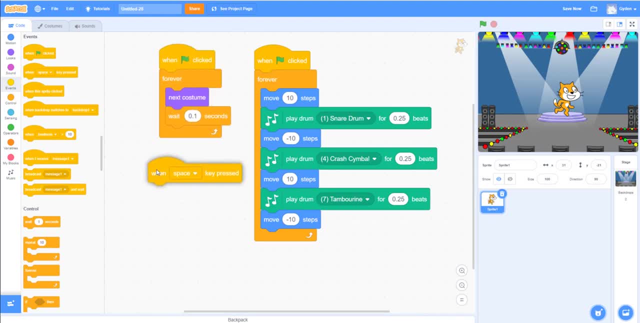 So when space keeps changing right, So when space keeps changing right. So here's: the key is pressed. so what we want to do is, when the space key is pressed, we want to change the color effect. So we're going to go back to look. 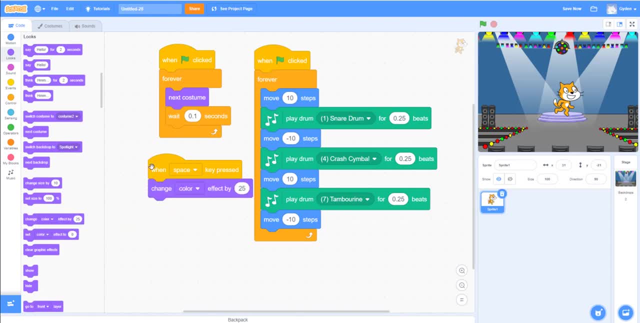 You can see that here changed color effect by 25. so what happened is? it kind of made the cat change the color and also you can make the cat say something if you like And you can say hello, right, And we can say hello for maybe 1 minute.